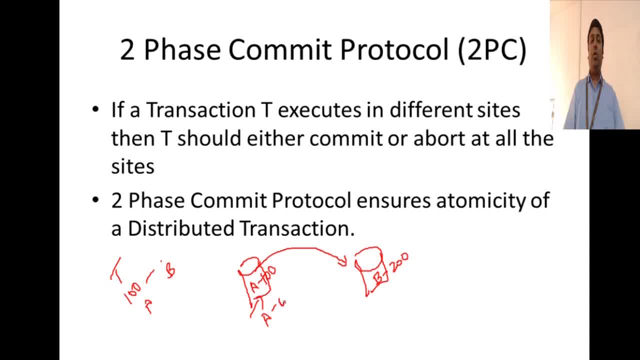 access this server, subtract 100 rupees here, so account A goes to 0. then I should go to this server, add 100 rupees here so that account B goes to 300. one single transaction executing at different sites, so that becomes a distributed transaction. What should be the property of this transaction? 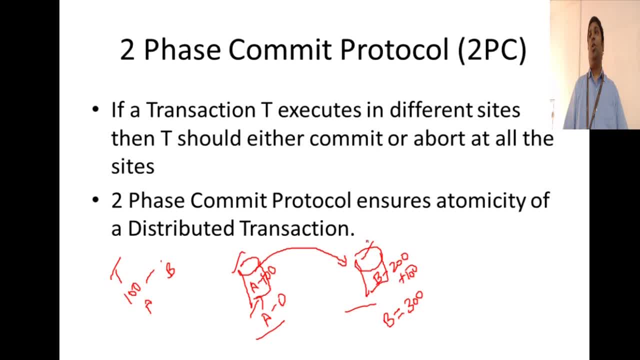 It should commit in both these sites or it should abort in all these sites. How will you ensure that this kind of a consistency or atomicity is established? You have to use a two-phase commit protocol. So today's class we are going to look at what is a two-phase commit protocol. 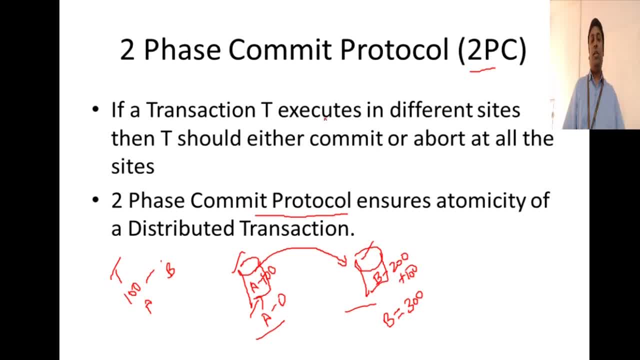 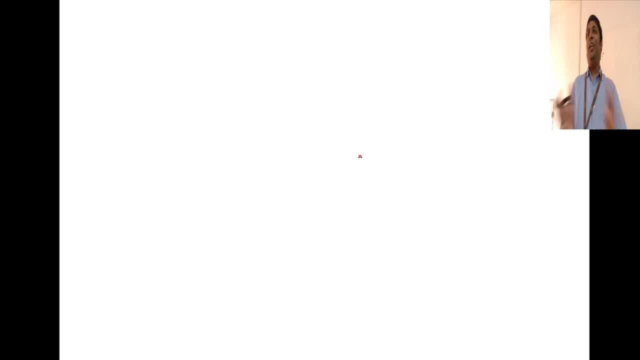 How it ensures atomicity of a distributed transaction. So I have got some animations for you. You can directly look at the animations and understand that simple protocol. So let me show what is this two-phase protocol. I mean two-phase commit protocol. Let us take 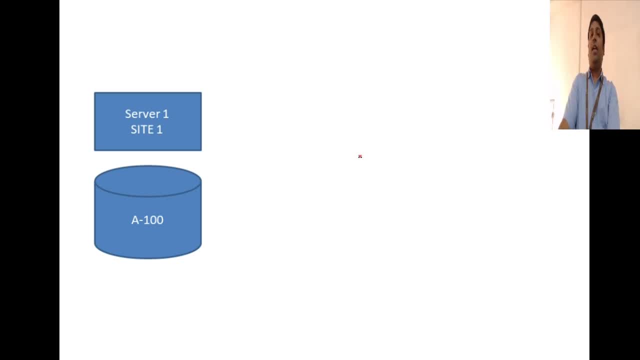 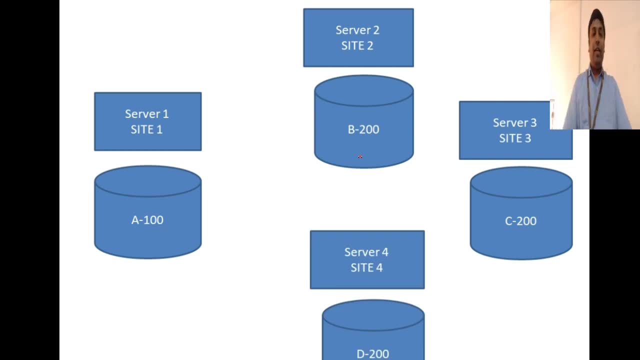 servers in different sites. Site 1, there is one instance running. site 2, another instance. site 3, site 4: 4 instances running and you can see here I have assumed some values. that is, here we have account A to be 100. 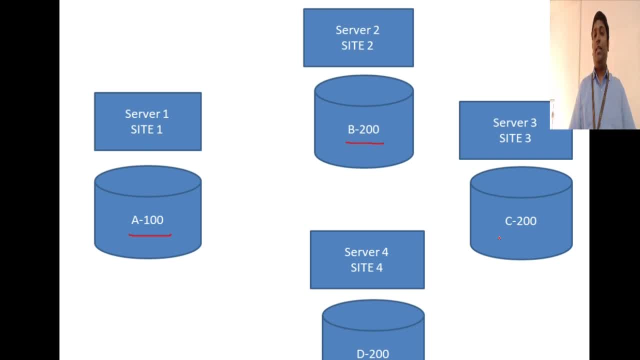 account B, value is here, that is, 200, account C is in site 3- 200, account D is in site 4, 200.. So we have 4 accounts distributed across different sites in a distributed system. Now let us say site 1. 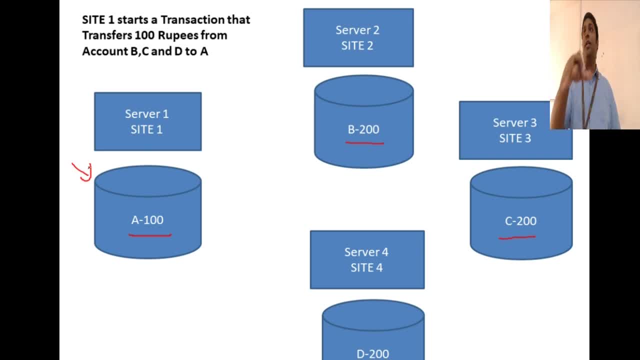 starts a transaction. A transaction will be initiated at one particular site. What is that transaction? I will transfer 100 rupees from all these sites to my account A, or what I can say is I will subtract 100 rupees from site 2,, site 3,, site 4. 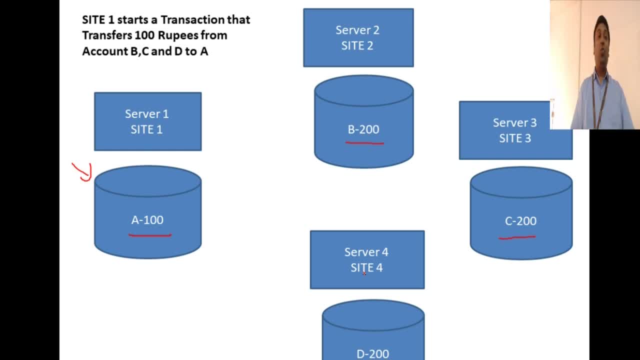 individually and add it to account A. So that is one single transaction. So this transaction will be executing on different sites, that is, site 1, site 2, site 3 and site 4, and I have given two boxes here Say this is the hard disk. 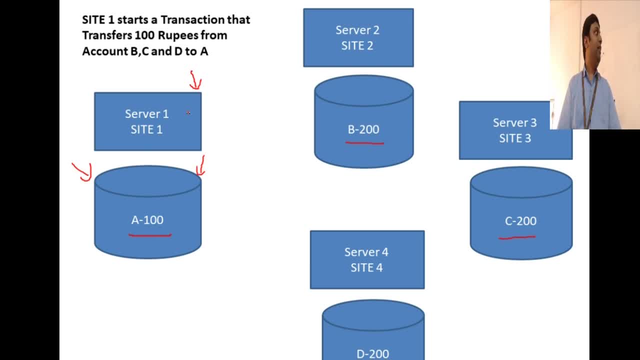 and this is the instance that is running. Maybe you can think of that to be the oracle instance running using the RAM. So this is an instance. If you are not clear about what is an instance, you can refer to my lecture on what is a database instance. 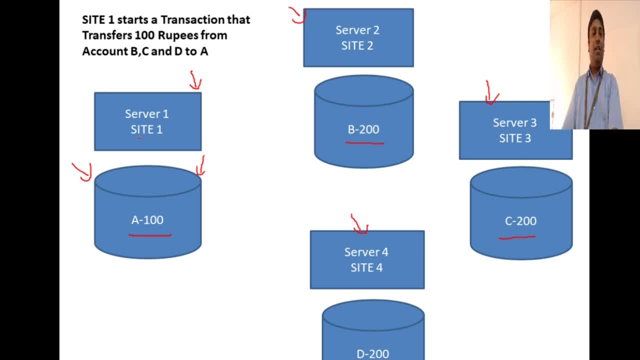 So now what happens is this transaction starts executing here, and what will be the process when a transaction starts executing? Say this: whatever content in the hard disk will be moved to your main memory and the processing will be done. So there will be a transaction manager. 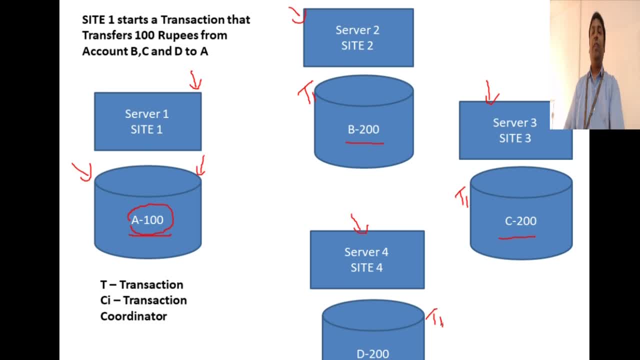 locally for every site. Every site will have its own local transaction manager. The site where the transaction originates will have the transaction coordinator. He will coordinate how these transactions execute in different sites And then the transaction starts processing, That is, it is going to subtract. 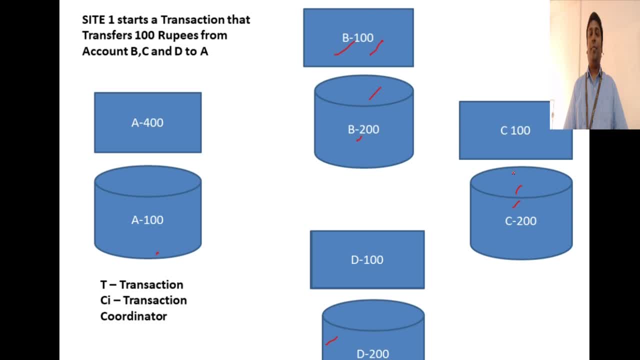 everything. Say, 200 is subtracted as 100,, 200 is subtracted as 100, 200 is subtracted as 100 in the buffer. So transaction executes on multiple sites. Likewise, 300 is added to A because we are transferring 100 from every account to A. So now, 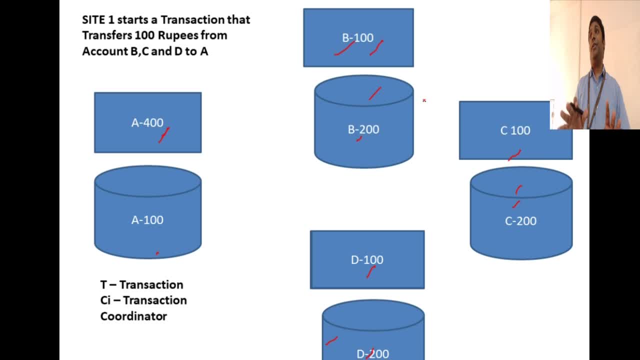 the transaction is executed, all its steps, in all these sites. This is when the two-phase commit protocol starts. We start with phase 1.. After all these steps are executed, we start with phase 1. What phase 1 does is you say: this is the transaction coordinator. 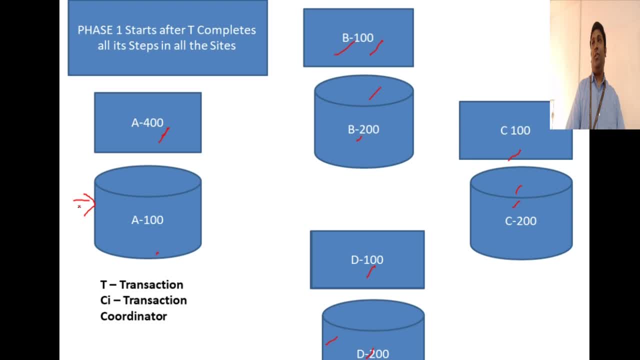 The transaction coordinator will send a message to all the participants. Who is the coordinator? He is the transaction coordinator. You call all these guys to be the participants in the transaction. So the coordinator, he will log a message And then he will send this message to all the participants. 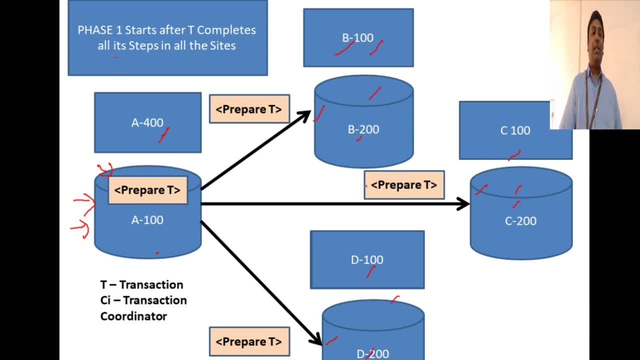 In phase 1. what happens? The coordinator logs a message on the stable storage. Okay, I am going to send a prepare message to all my participants. So this will be moved to the stable storage on the hard disk And this message will be sent to all the participants in the transaction. That is. 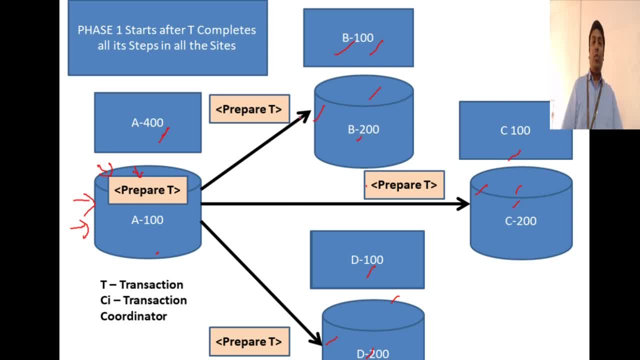 happening in phase 1.. Once when all these servers receive this message, the next step, what they will do is they will log a ready message. That is, they will log a ready message to their hard disks: Okay, we are all ready to commit, That's the meaning. So they will put that. 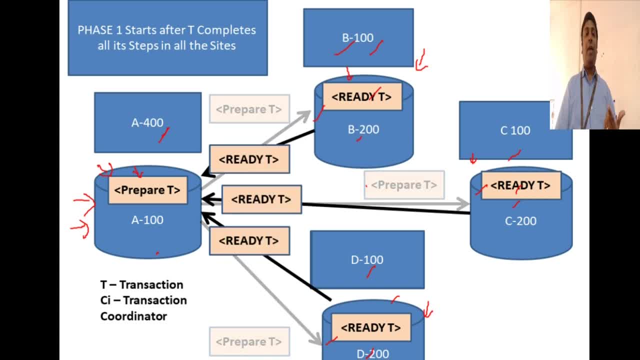 message in their hard disk and then transmit that message back to the coordinator. We are all done, We are ready to commit. That is the meaning of this. The coordinator will receive all the ready messages from every participant. Now phase 2 starts. 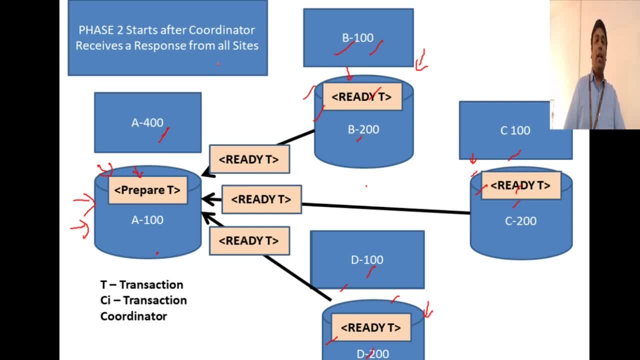 After the received of the message, we have phase 2.. What happens in phase 2 is the coordinator will check whether it has received ready message from all the participants. If it has received ready message, then what it does is it will log a commit log and then it will send a commit message to all the participants. 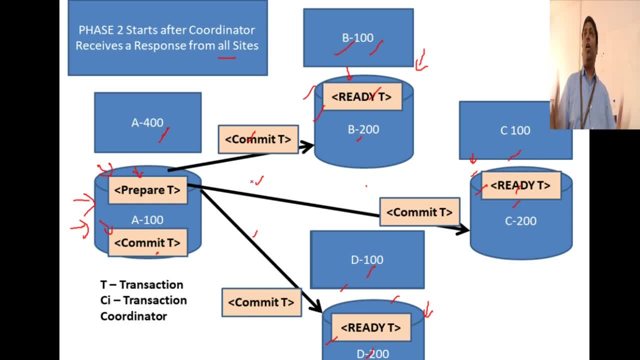 Since everyone said we are ready, what the coordinator will do: send a commit to all the participants. The participants will also log this commit on the hard disk and then they will change the data. So this is the phase 2.. So this is two phase commit protocol, And now we will see. 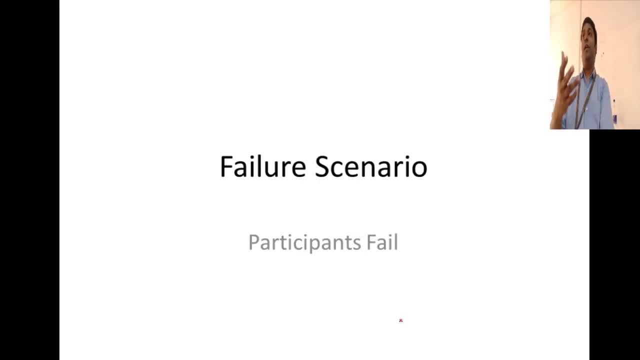 failures. What kind of failures can happen during a transaction? How it recovers. The first kind of scenario is participants failing. What happens when a participants fail? So let's again go to the same scenario. We have servers, We are going to perform. 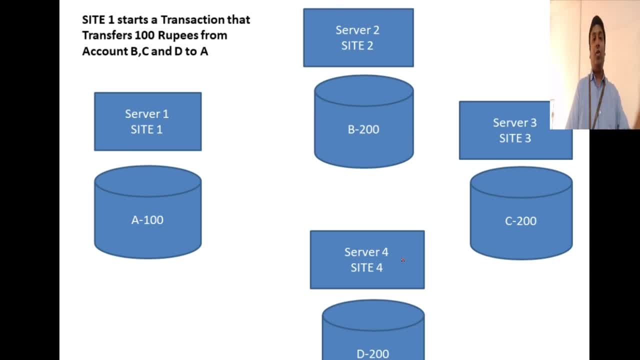 the same action. Move 300 rupees from all these accounts to account A and everything gets changed. The buffer gets changed. Now everybody is ready. Now what happens is the coordinator is going to send a prepare message, as usual. You log it and send a prepare message to all the participants. 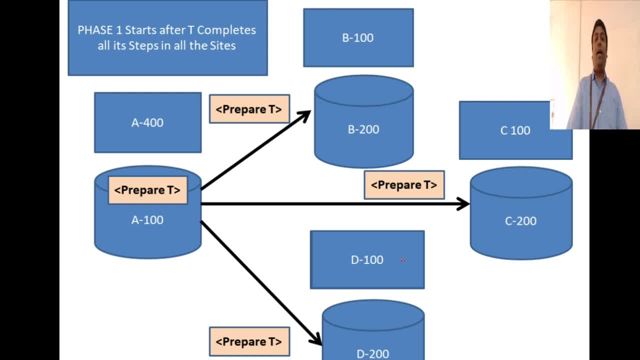 Now what happens is the participants should send a ready message after logging it. So say participant sends a ready message, but before that they will log it. So this participant is logging a ready message. Likewise, this participant is logging a ready message And this participant fails. 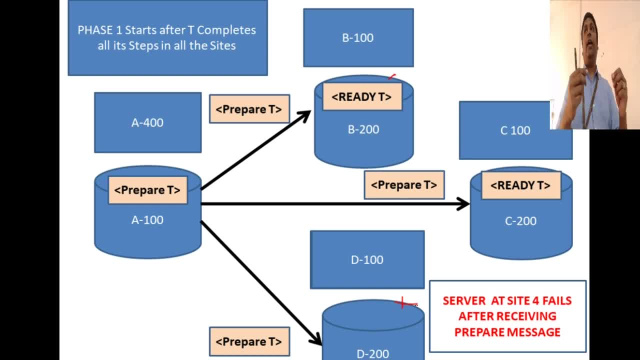 Maybe he crashes down or he enters into a network issue. So what happens? the remaining participants will send the ready message back to the coordinator, But this participant will not send a ready message back. The coordinator will know something is wrong because he didn't get the ready message from all the participants. So what now? the 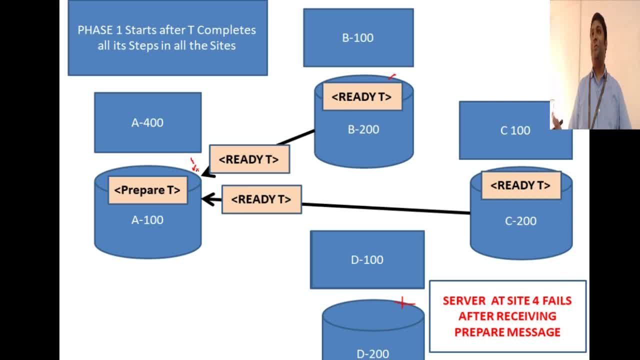 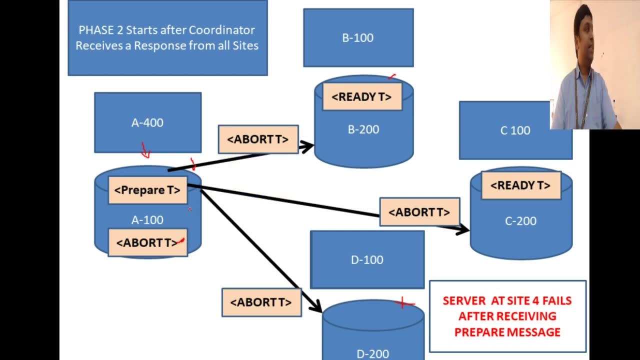 coordinator should do. The coordinator should cancel the transaction Because one of the sites failed. So what the coordinator does is he will log an abort and then send an abort message to all the sites So that all these sites cancel the transaction, Cancel the. 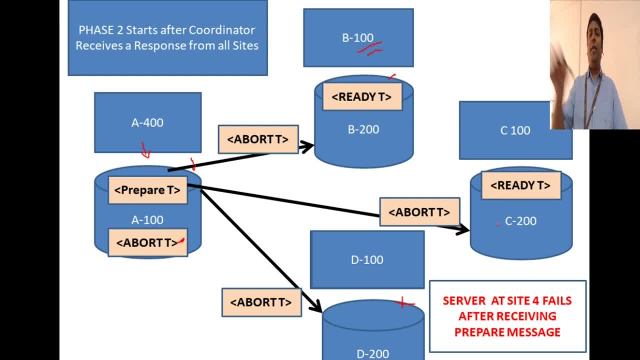 transaction. in the sense, none of the changes in the buffer will be impacting the hard disk, So our change is nothing to undo. then This happens when a particular participant fails to send a ready message back to the coordinator. Failure scenario 2.. Participant fails. 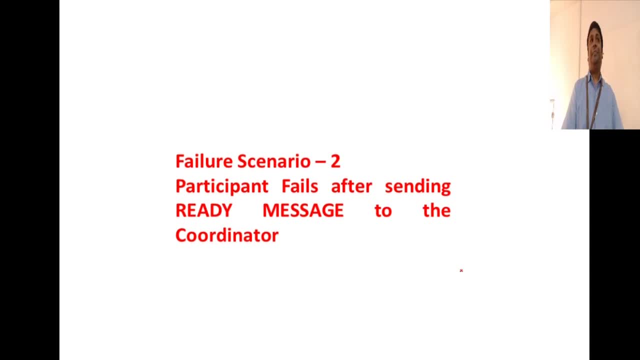 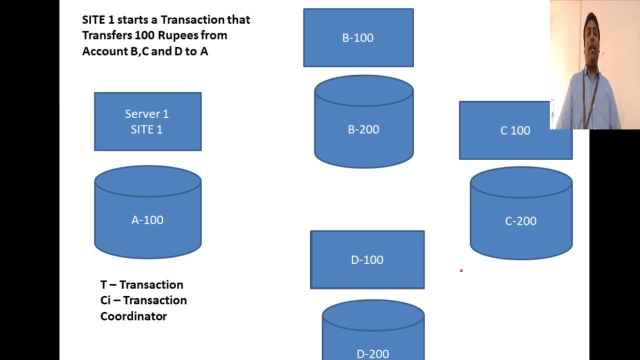 after sending a ready message. What happens when a participant fails after sending a ready message? So he will repeat the same process and everybody has changed their contents in the buffer. Coordinator now sends logs a prepared message and then he sends the prepared message to all the sites. 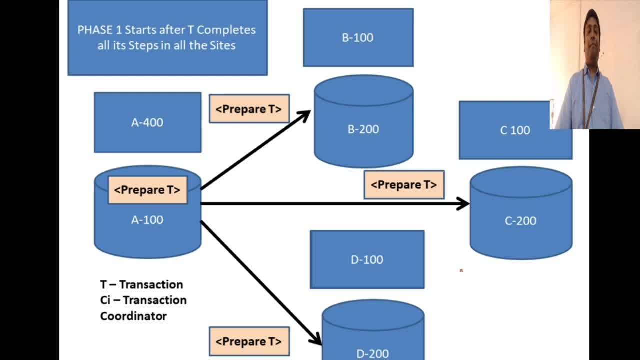 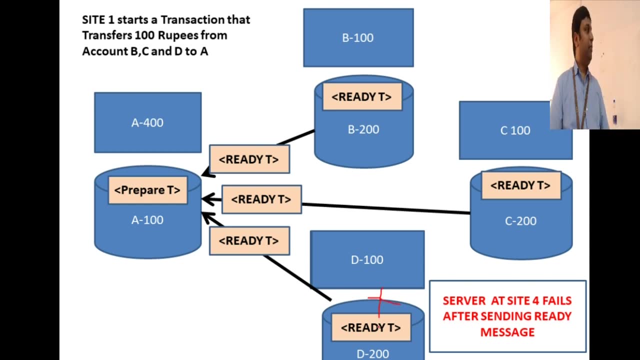 So once when the participants are ready- everybody is ready, right- they will log a ready message in the hard disk and then send a ready message back. After sending a ready message, this guy fails. What do you mean by a failure? He can end up in a network issue. he can. 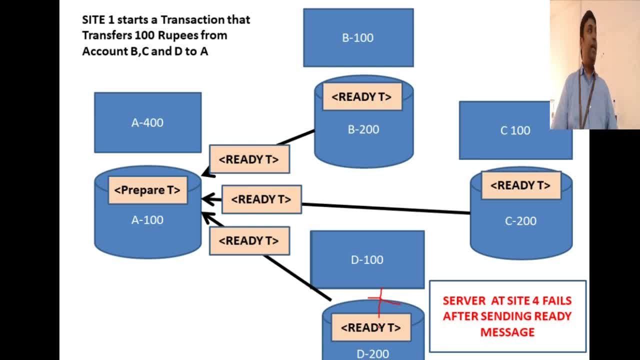 crash down, some disk failure can happen, anything can happen. But he has sent a ready message and he failed. So now this coordinator what he will do. he knows that everybody has sent a ready message, so he is going to go and log a commit record and then send a commit message. 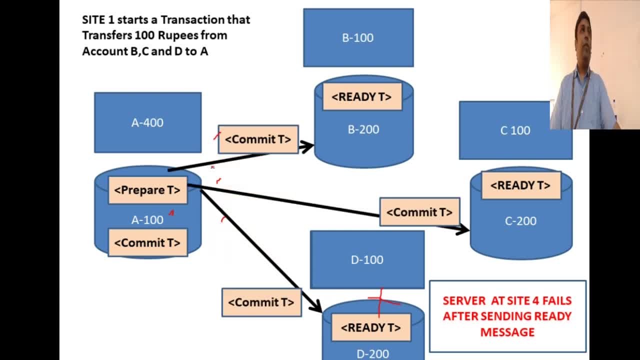 to all the participants. He is not worried who has failed because since he got a ready message, he just sends commit. So this guy will not receive anything. he is down. The other two guys will receive a commit and then what they will do? they will log this commit record. 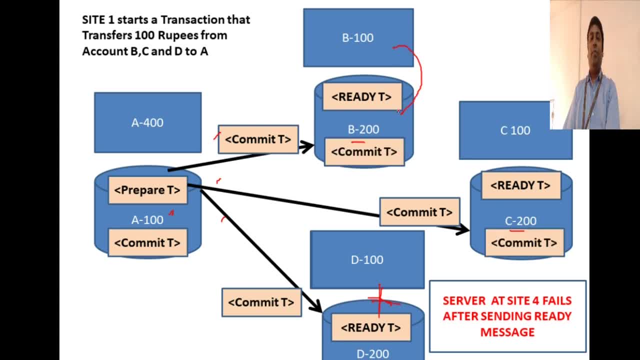 first, and then they will go and update the changes in the buffer to the hard disk. So changes happen in two of the sites, whereas this site is down and he is not even able to get that commit message. So what happens is this site will recover, in the sense whatever that is down will. 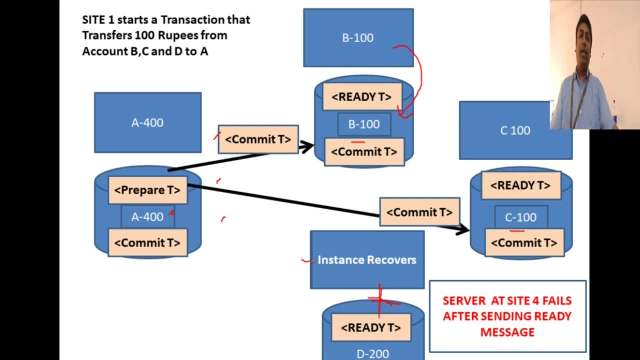 recover. Maybe we reboot it, we start it again. the site recovers, but it is unsure what happened. So how this should be fixed is this site should contact the coordinator to see what happened. The coordinator will know the transaction committed using its. 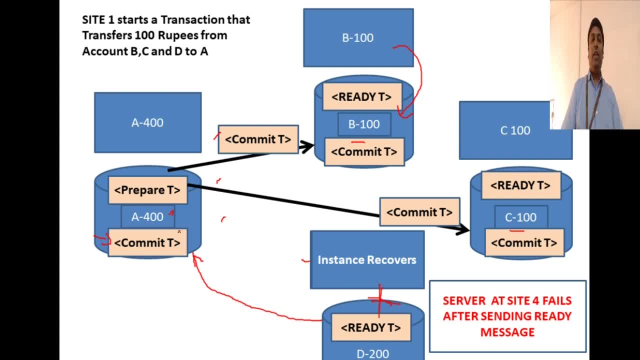 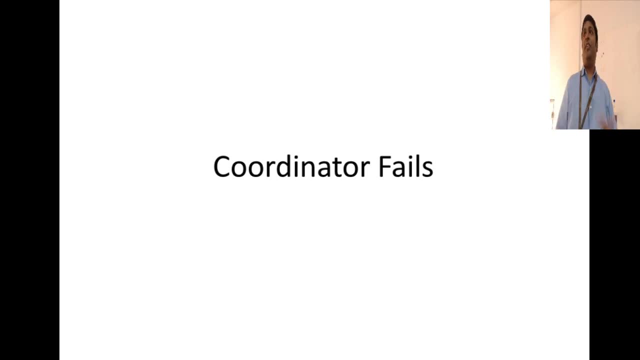 log file. So this information will be passed to the participant so that this guy can go and apply the changes to his database. Now we will take another failure scenario: coordinator fails. What do you mean by coordinator failing? and we will take one scenario here. 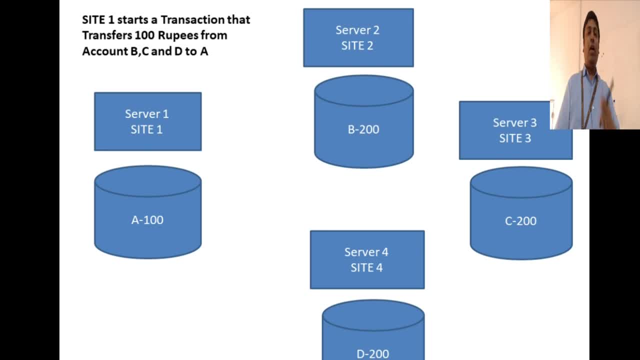 Again, 4 servers, the same concept. move 100 rupees from every account to your account A and the transaction does all these steps. Phase 1 starts. What is that? Coordinator logs a prepare message into the stable state and then sends the prepare message to all the participants. 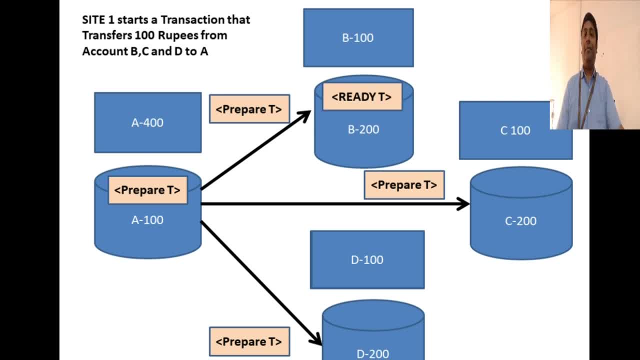 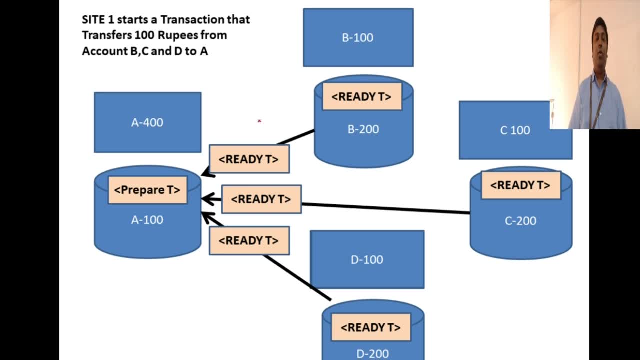 Now participants are ready, Say they log a ready message and then they send the ready message back to the coordinator. When the coordinator receives the ready message it will know: right, everybody has sent a ready message. What is the next step? Log a commit and then 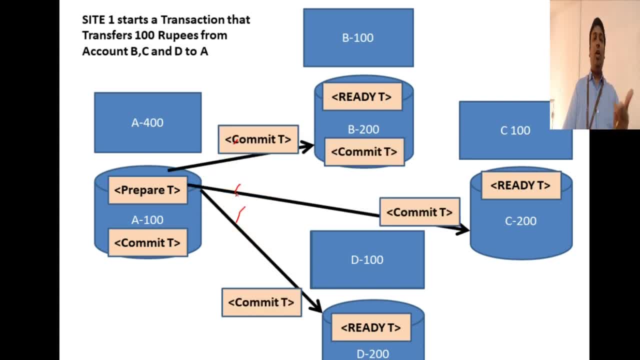 issue a commit to all the participants. So participants will log this commit. After logging the commit record, they will be moving the changes to the hard disk. So everybody moves the changes to the hard disk. So everybody has done it right and they have done the commit. and now coordinator. 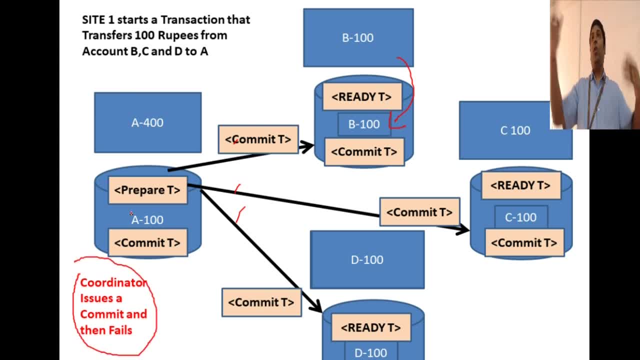 fails. See, coordinator sends a commit to everybody and coordinator fails, So will there be any issue? What should coordinator do? He should also log this 400 to the hard disk, right? He has issued a commit, but then he has failed. So when he 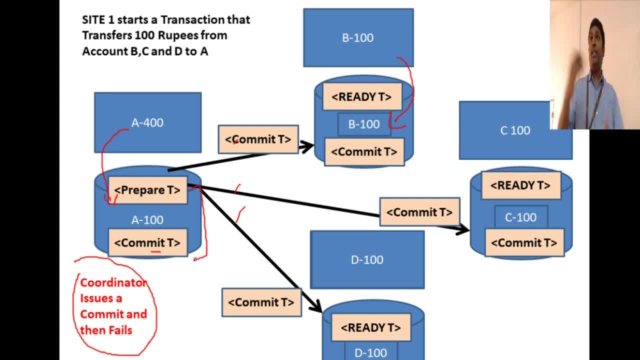 recovers. what he will do? he will go to the log files. He knows that the transaction has been committed, so he will just apply the changes to the database so that it goes to 400. So everything happens. recovery happens using log files. 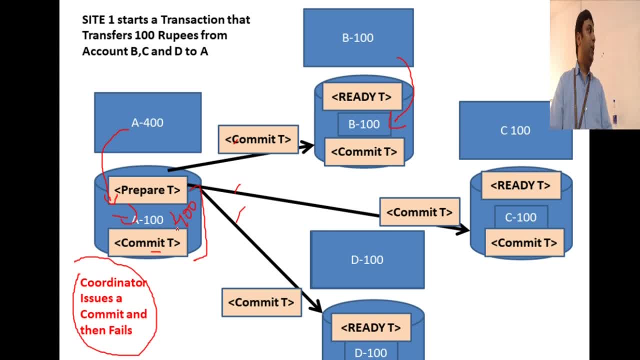 So that is the scenario wherein a coordinator fails after sending a commit message. So the coordinator will recover using the log files. he will go and apply the changes. If you are very unsure about what are recovery techniques, I have given a detailed lectures on all the recovery techniques for database. 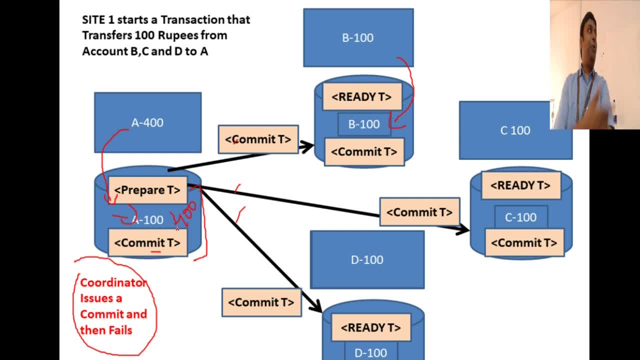 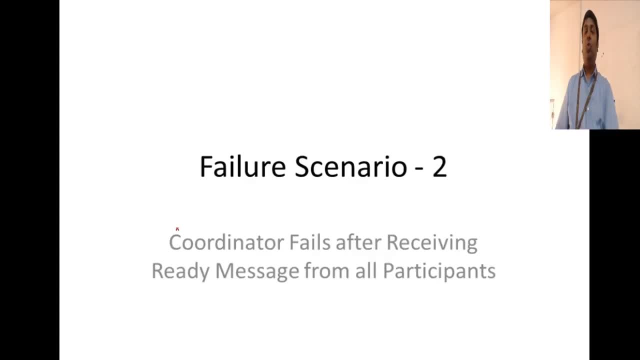 management systems for VTech students. You have to go and refresh that to understand this in depth. Failure scenario 2.. This is the most important scenario. Coordinator fails after receiving ready message from all participants. We will take a look at this scenario. 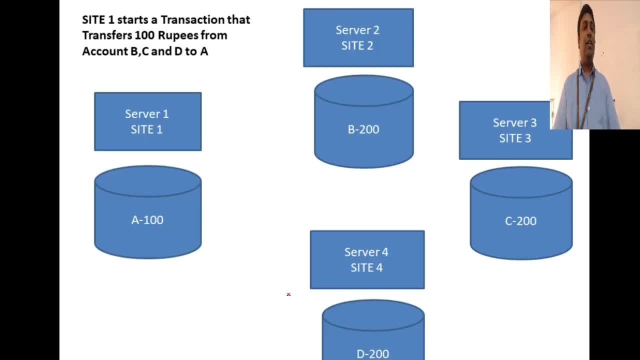 Again we have these 3 or 4 sites. The operation of the transaction is transfer 100 rupees from every site to site 1.. So this is the coordinating site. So, as usual, this guy will log in a prepare message once the transaction completes all the steps. This: 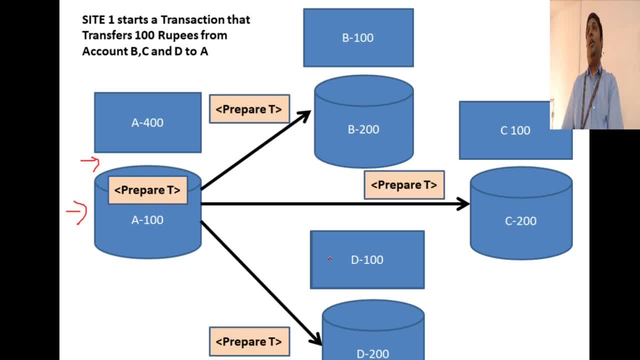 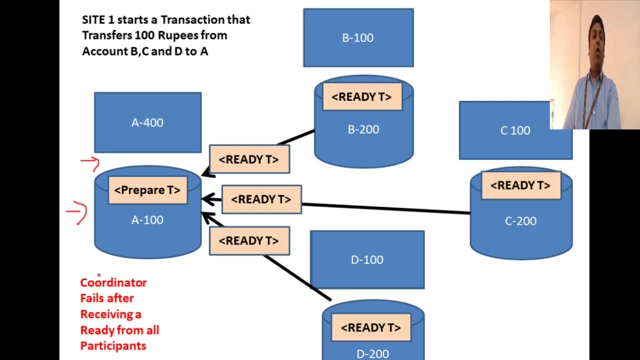 coordinator will log in a prepare message, send that message to all the participants. Participants will now log a ready message and then they will be sending a ready back to the coordinator. So at this instance, when they send a ready back, the coordinator fails. 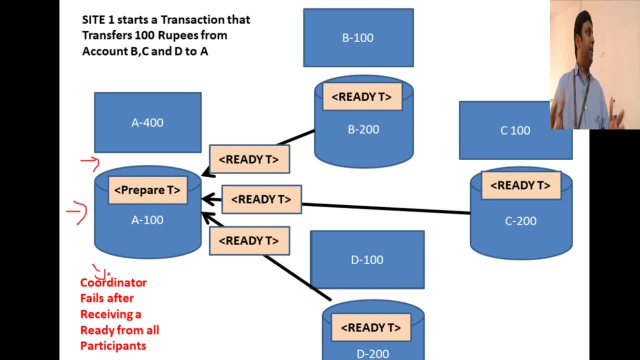 Everybody has sent, we are ready. The coordinator received the messages and then it crashed. So now how to recover? Unless the coordinator sends a commit, all the others will be waiting. So what happens when you run transactions? you are going to apply logs. 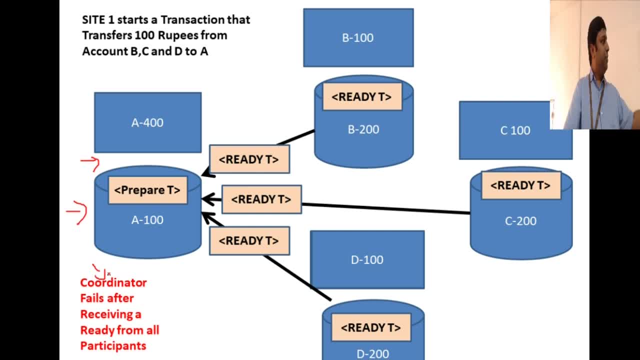 whole database items. So all these independent servers will be locking items and then they will be waiting for the coordinator to send a commit. But coordinator has failed. So what is the only option available here is the coordinator should recover and then he should send a commit message to the participants. What is the drawback? 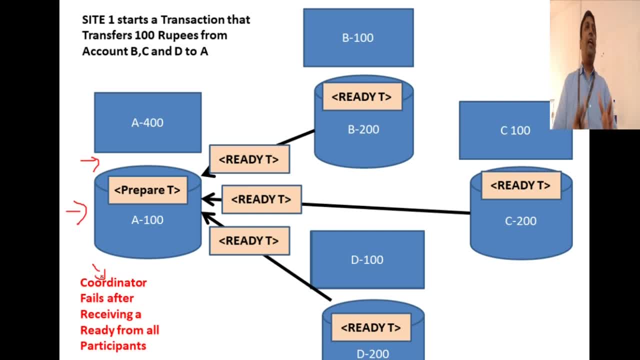 of this Till the coordinator recovers and sends a commit message. every participant will be waiting for the message. They will be locking the items and then waiting. So that is called blocking of resources. I mean the participants are locking the items and locking the resources till the coordinator recovers and sends. 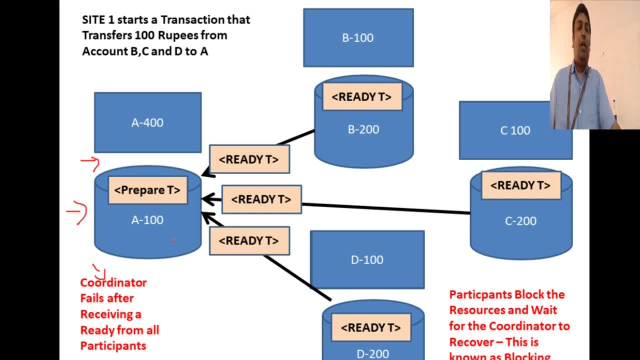 a commit message back. So that is how the failure scenarios are handled in a two-phase commit protocol. What is a two-phase commit protocol? In phase 1, I log a prepared message, send it to my participants. Participants will send a ready message if they are ready to commit. In phase 2. 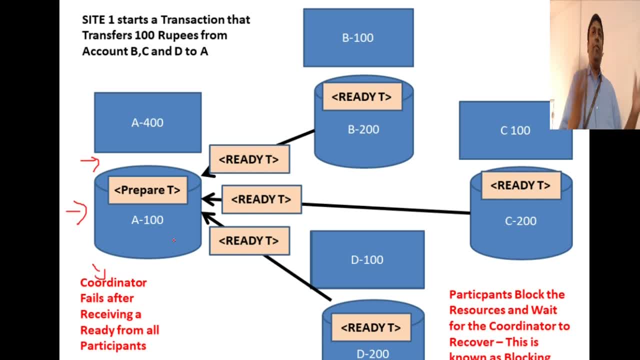 the coordinator will check whether everybody has sent a ready message. If everybody has sent, it will send a commit message to all the participants. Everybody will commit. If one of the participants is not replying with a ready after an elapsed time, the coordinator knows I did not get one of the ready messages, So it will send an abort to. 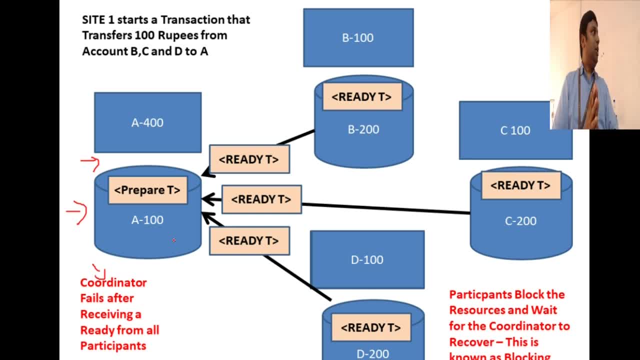 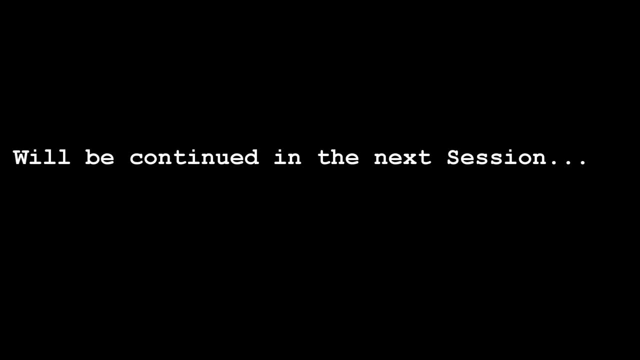 all the servers, Everybody will abort. So this is how two-phase commit works in a distributed environment. So that is how two-phase commit works. So this is how two-phase commit works in a distributed environment. Now let us move on to the next phase. So now the two-phase commit works. 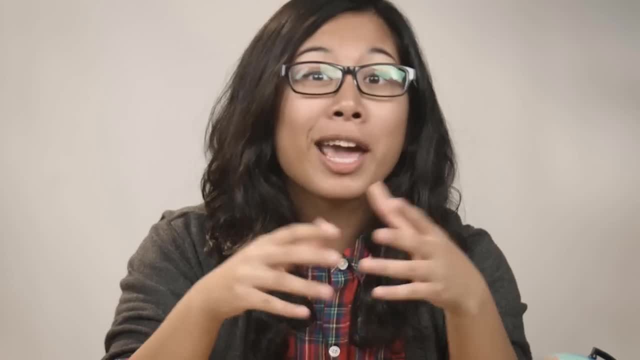 Hey, what's the difference between weather and climate? You can't weather a tree, but you can climb it! 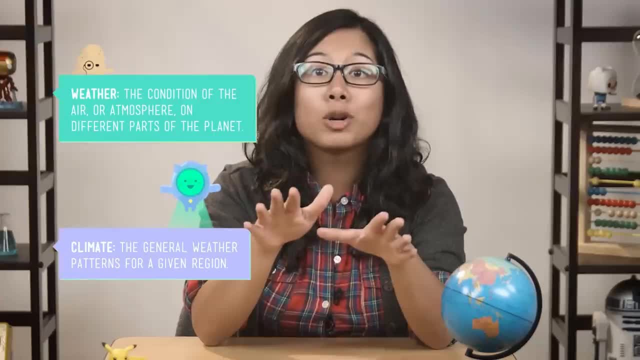 But you already know the difference between weather and climate. And if it slipped your mind, psst, the definitions are right there. 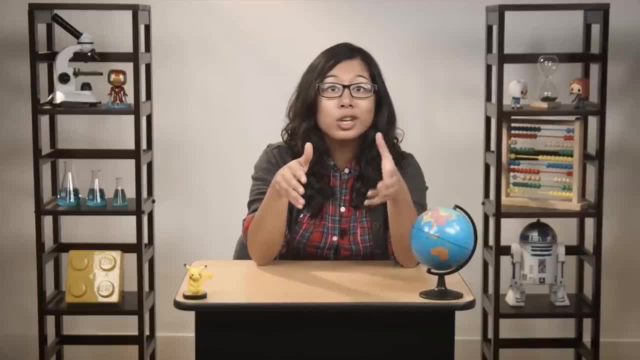 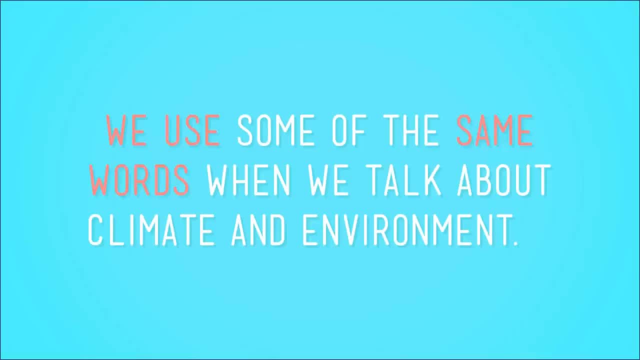 You know that the weather can change quickly, but climate can also change, just more slowly. And if you're good at putting two and two together, and I know you are, you probably already noticed that we use some of the same words when we talk about climate and environment. Words like temperature and rainfall. Coincidence? I think not. 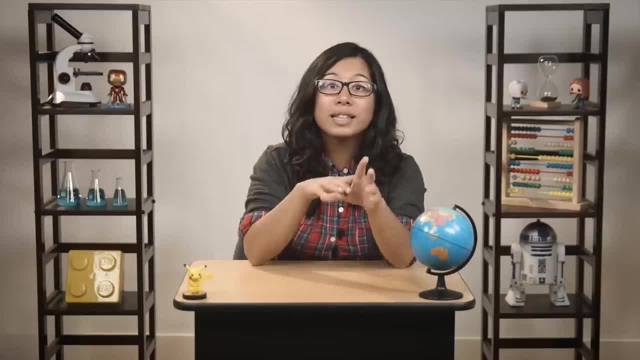 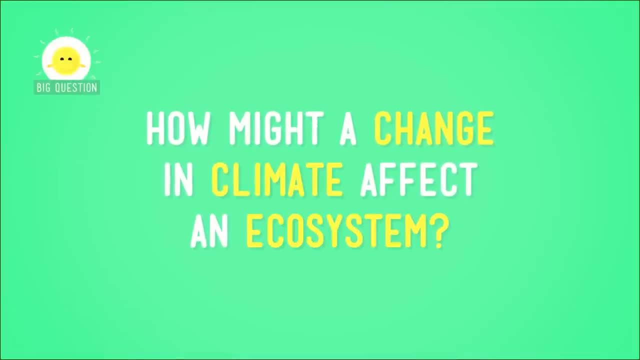 But science demands evidence, my friends. And while we've already seen that living things can change when environments change, we need to ask, how might a change in climate affect an ecosystem? 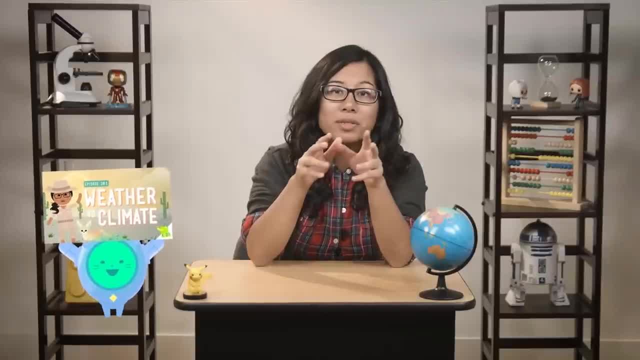 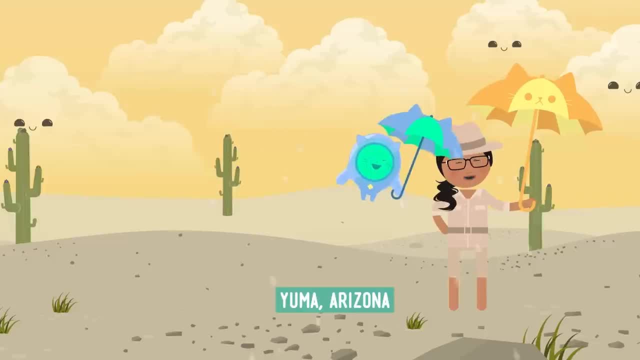 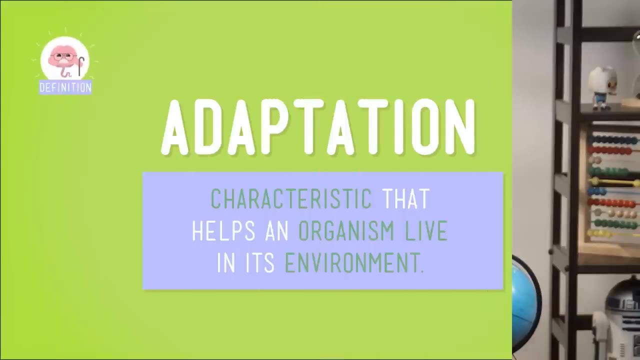 First, let's talk climate. Through Little Me's travels, we found out that Yuma, Arizona had a hot and sunny climate. We decided this after finding out that, although it rained once or twice during my long stay, most of the days were hot and dry. Now, the plants and animals that live in Yuma's hot, dry, sunny climate have adaptations that help them live in that desert environment. 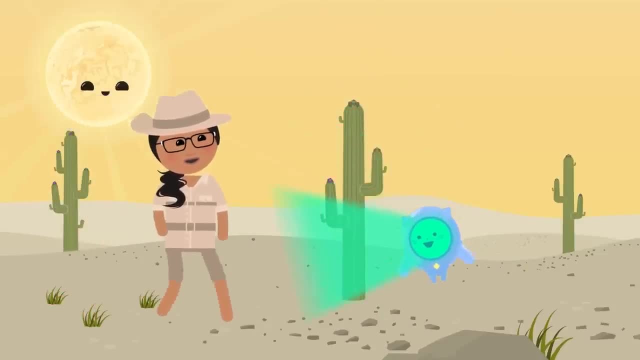 If we took a hike around Yuma, we might see a cactus, and if we took a closer and careful look at the cactus, we'd see that its outside is kind of waxy and tough. Now, say something happened to Yuma's climate. Say, over the course of about 20 years, there were even hotter days and less rainfall than before. When weather patterns change over a long period of time, we call it climate change. 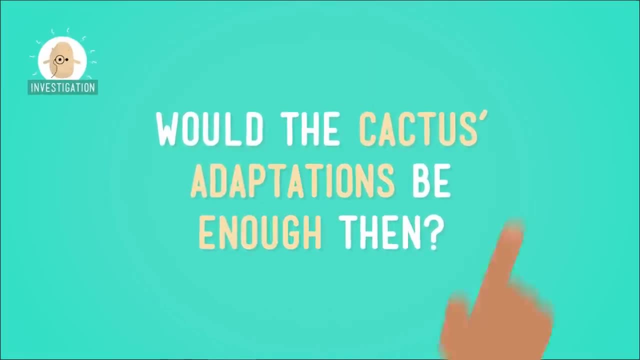